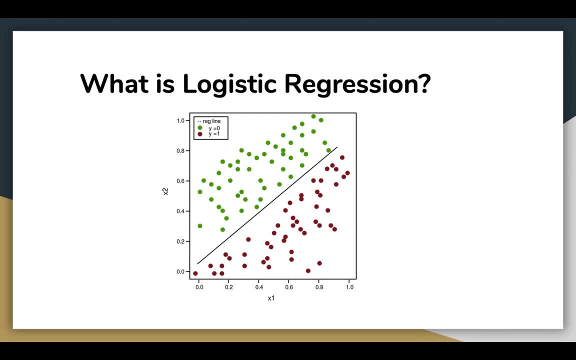 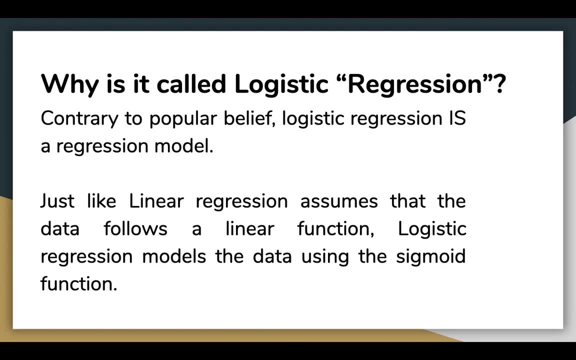 As we can see here, we need to categorize the data in two different categories, and our job is to define the line which does that. Now, why is it called Logistic Regression if it is a classification mechanism? Contrary to popular belief, Logistic Regression is a regression model. The model builds a 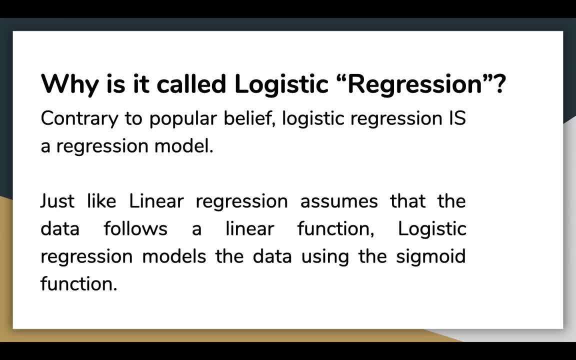 regression model to predict the probability that a given data entry belongs to the category numbered as 1.. Just like linear regression assumes that the data follows a linear function, Logistic Regression models the data using a sigmoid function. Linear regression gives you a continuous output. 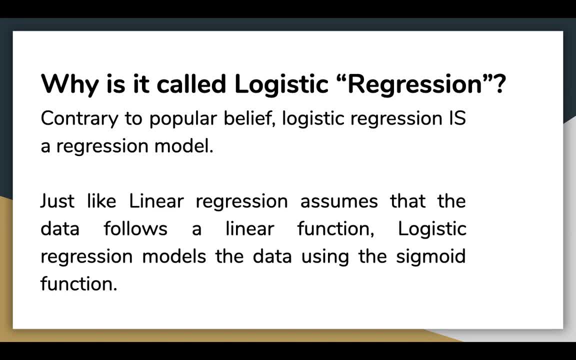 Logistic Regression models the data using a sigmoid function. Linear regression gives you a continuous output, But Logistic Regression provides a constant output. An example of continuous output would be house price prediction or stock price prediction. An example of discrete output is predicting whether a patient has cancer or not, or predicting whether a customer will click on an ad or not. 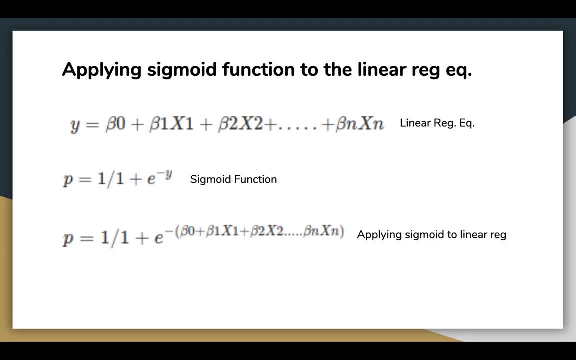 Now let's modify the linear regression equation we had seen in the previous video. for logistic regression, We apply something called as a sigmoid function on the linear regression equation. Let's see what the sigmoid function is. Let's see what the sigmoid function is. 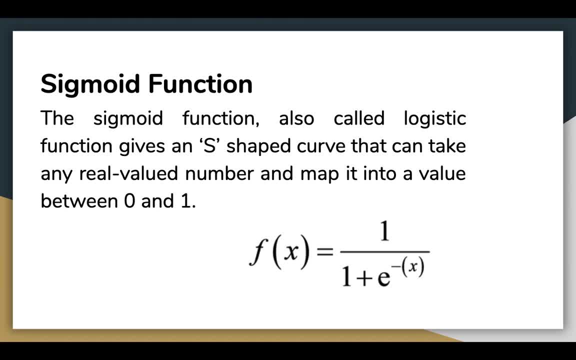 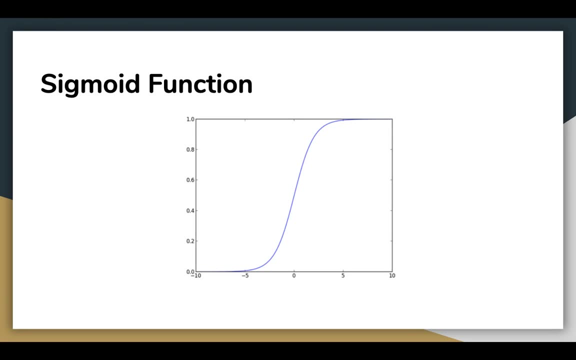 Let's see what the sigmoid function is. The sigmoid function, also called the logistic function, gives an S-shaped curve that can take any real-valued number and map it into a value between 0 and 1.. If the curve goes to positive infinity, y predicted will be 1. and if the curve goes, 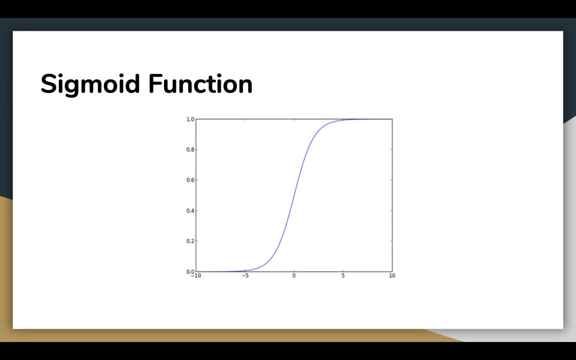 to negative infinity, y predicted will become 0.. If the output of the sigmoid function is more than 0.5, we can classify the outcome as 0.5.. We can classify the outcome as yes or a 1, and if it is less than 0.5, we can classify. 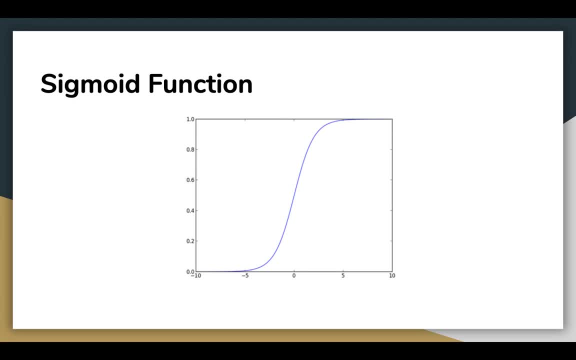 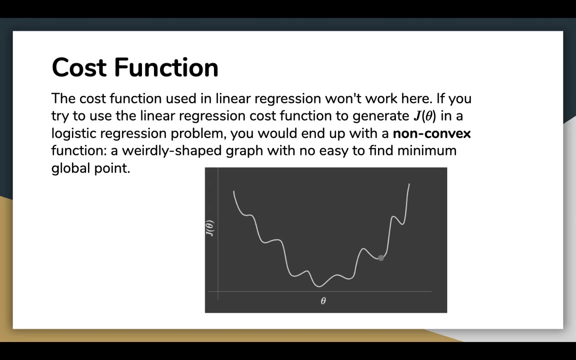 it as 0 or a no. For example, if the output is 0.75, we can say in terms of probability, as there is 75% chance that patient will suffer from cancer. Just like we have a cost function in linear regression, we need one for logistic regression. 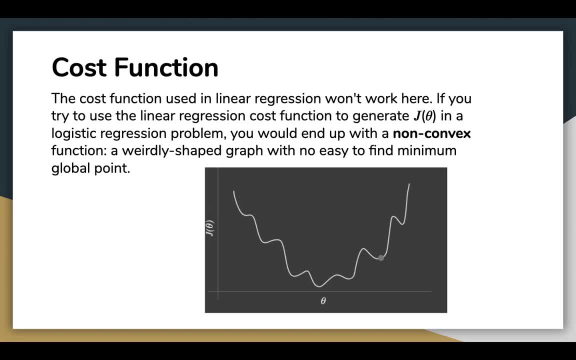 as well, which has to be reduced to obtain the best fit line. But the cost function used in linear regression will not work here. If you try to use the linear regression cost function in a logistic regression problem, you would end up with a non-convex function, a weirdly shaped graph with no easy way to.